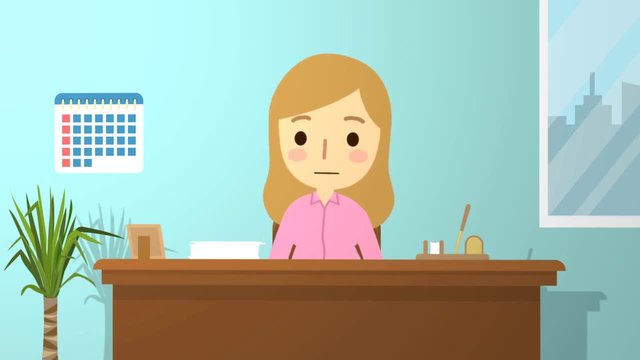 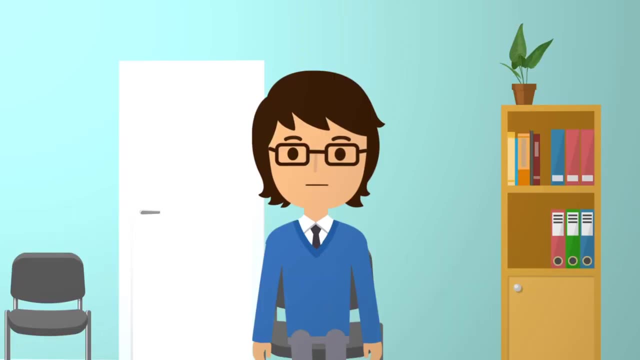 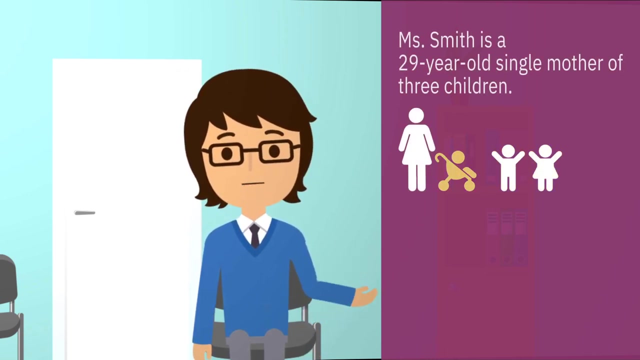 Great Thank you. You were assigned this case for investigation a few days ago. Can you tell me about the family and the most recent allegations you investigated? Well, Ms Smith is a 29-year-old single mother of three children: A 9-year-old, a 7-year-old and an infant. 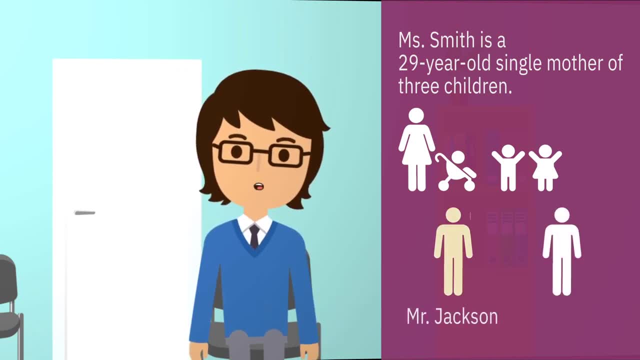 There are two different fathers in this case. Jim Jackson is the father of the infant and is currently incarcerated. Brian Martinez is the father of the older children. Ms Smith and Mr Martinez are both drug addicts and have a long history of Child Protective Services involvement. 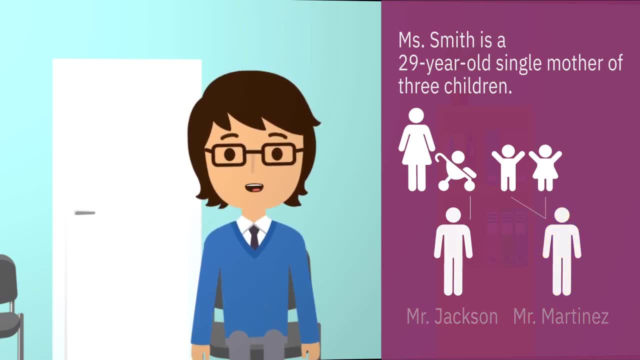 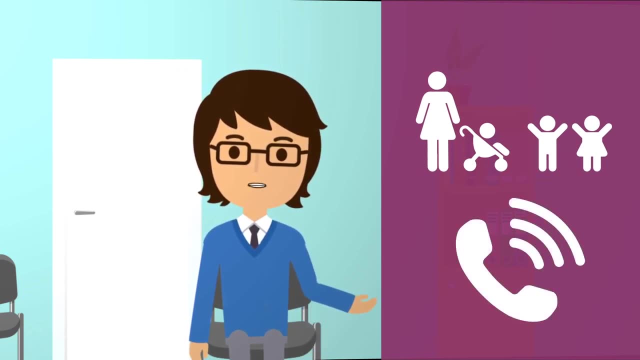 Mr Martinez has not been in the home nor parented his children in a long time. A few days ago, a report on this family was received by the hotline And after my full investigation, I conducted an emergency removal of the children because they were unsafe and in immediate danger. 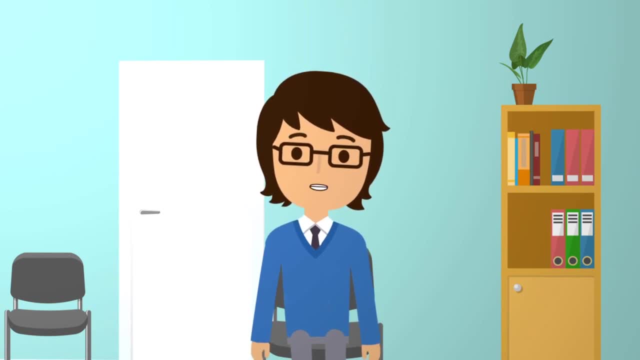 You might recall some of the details from our staffing at the time of the children's removal, so let me know if you want me to provide more details as I go. Thank you, Please continue. Okay, As I said, the children were removed due to multiple safety and risk factors. 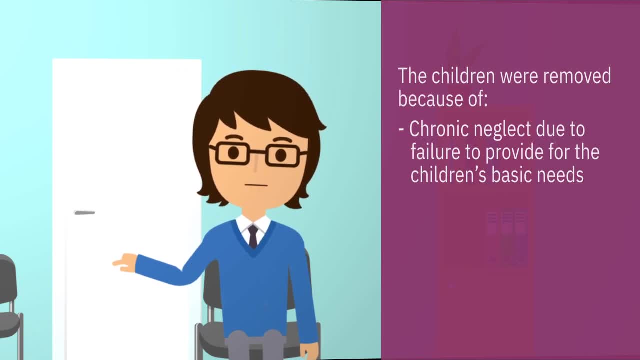 First, there were substantiated allegations of chronic neglect because of mom's failure to provide for the children's basic needs, as well as substantiated allegations of inadequate supervision of the two older children. The older children were left at home alone for hours at a time, often with limited or no food. 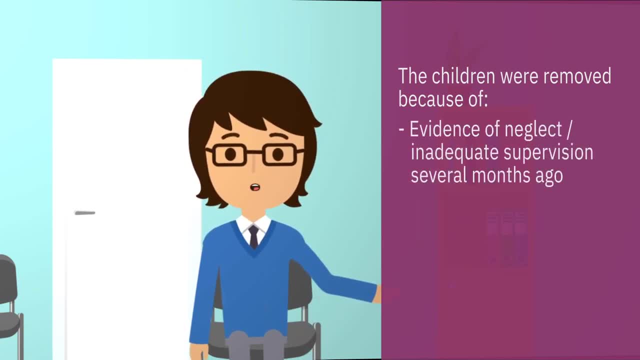 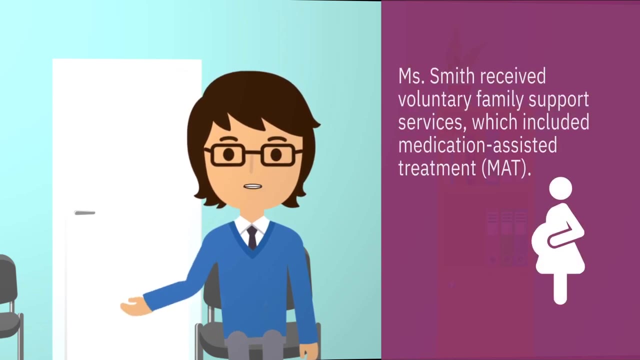 Second, several months ago there were allegations of neglect that were substantiated. The findings of neglect were inadequate supervision. Also, we received a report of physical neglect of the infant who was born with prenatal exposure to methadone. During her recent pregnancy, Ms Smith received voluntary family support services. 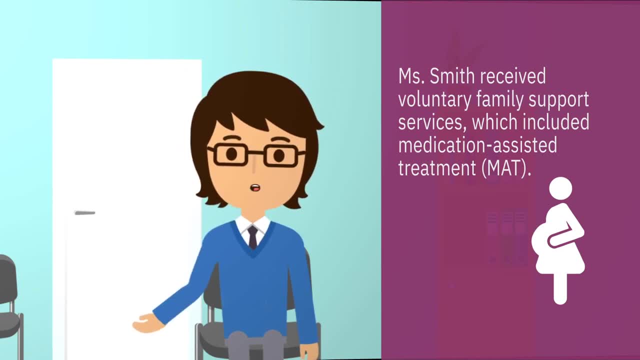 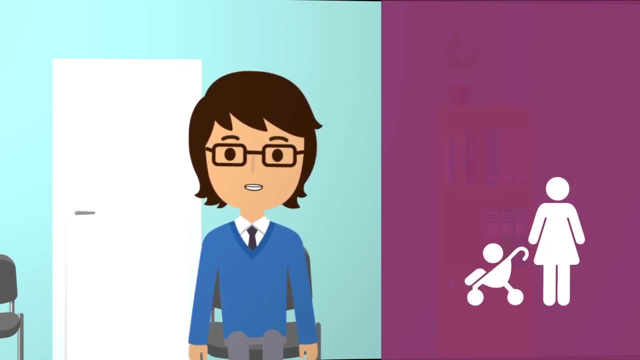 and she was able to provide for the children. The report included medication-assisted treatment for her addiction. The voluntary case was closed only four weeks prior to Ms Smith giving birth. When the baby was born, the mother and child both tested positive for methadone. 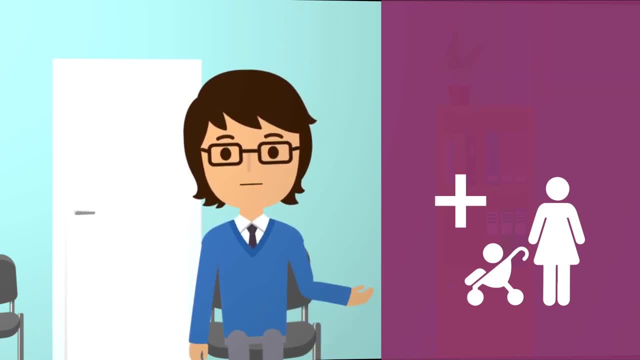 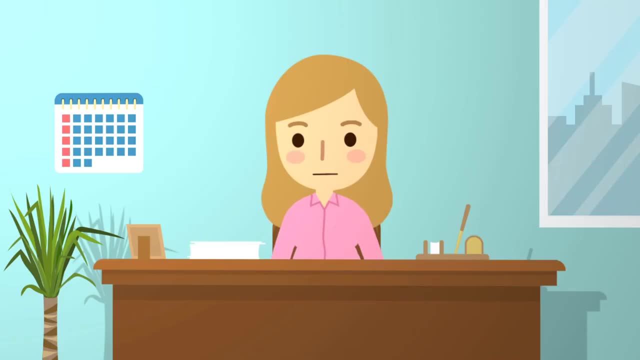 and the hotline received a report. In the voluntary case plan, the ongoing worker recommended that Ms Smith discontinue methadone treatment. Okay, So far. I understand the allegations and findings. Ricardo, Please continue, but I would like to read the report. 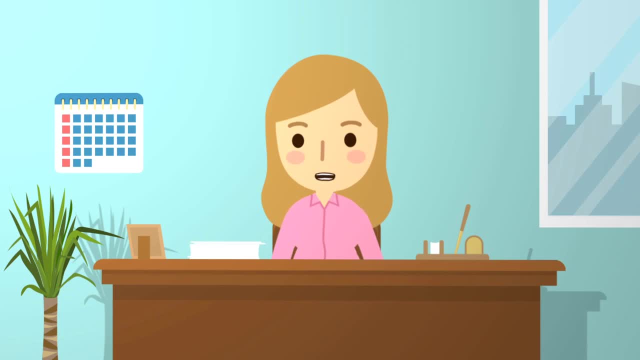 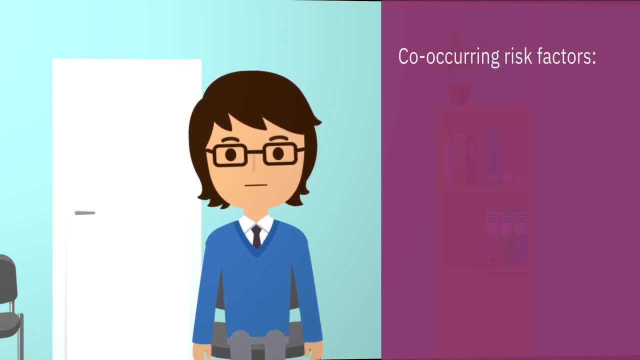 I would like to revisit why our department recommended Ms Smith discontinue methadone during her pregnancy. There were co-occurring risk factors that increased the children's vulnerability to maltreatment, including chronic substance use in the home, lack of family support, the child's age. 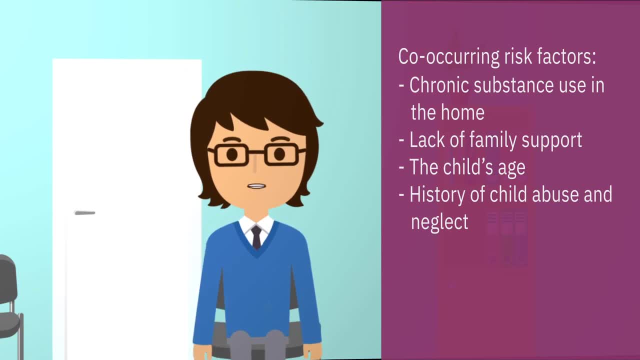 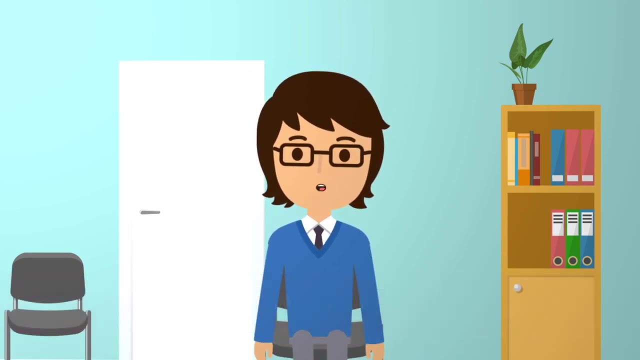 and an extensive history of child abuse and neglect. Plus, Ms Smith recently participated in the voluntary case that I just spoke about, but she stopped her involvement in services. The recent investigation produced substantial evidence that warranted ongoing CPS involvement for this family and the filing of a dependency petition to place the children into care. 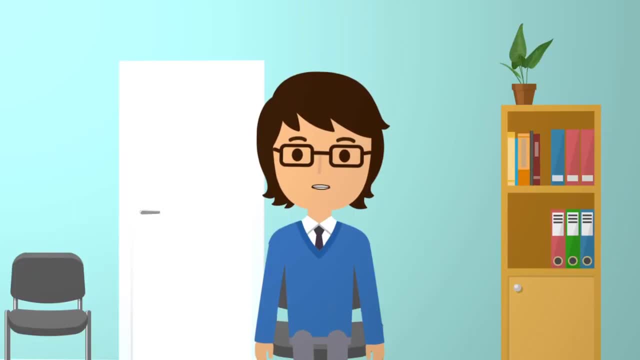 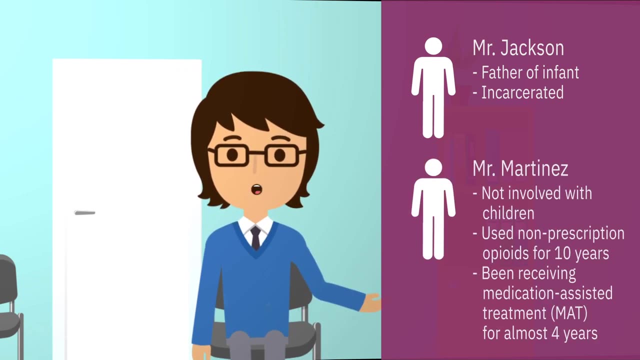 Can you give me more information about the fathers? Yes, As I mentioned, Jim Jackson is the father of the infant and is currently incarcerated. Brian Martinez isn't involved with the children. Mr Martinez previously used nonprescription opioids for 10 years. 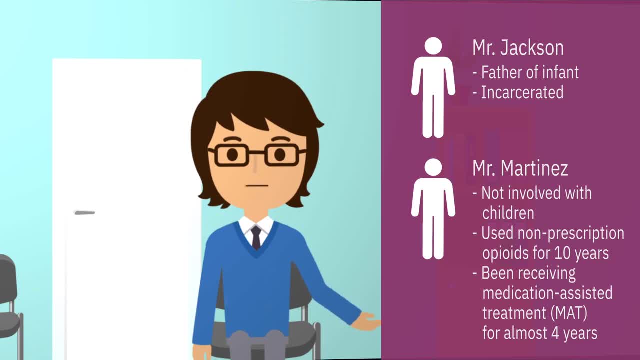 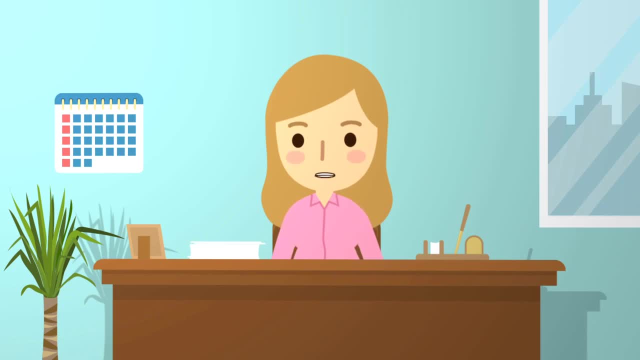 and has been receiving MAT services through an evening outpatient treatment program for almost four years. Is there any evidence that the child is currently incarcerated? Is Ms Smith currently receiving services to treat her substance use disorder? Yes, Ms Smith provided the information from her MAT outpatient program. 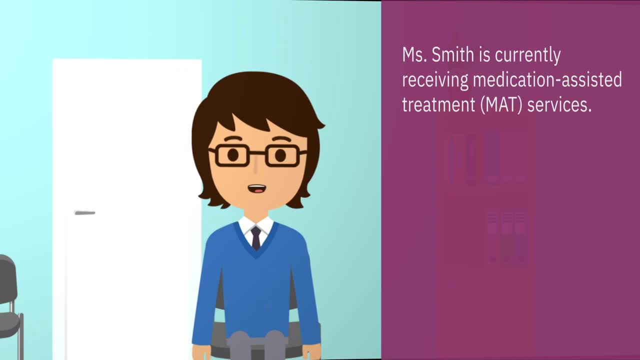 and the individual counseling services she attended. I contacted the program and Ms Smith discontinued the counseling services, So her voluntary case with Kara was closed. Ms Smith never discontinued the use of methadone during her pregnancy, as her ongoing caseworker, Kara recommended. 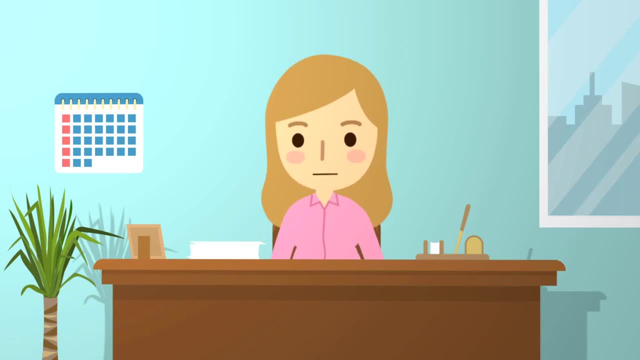 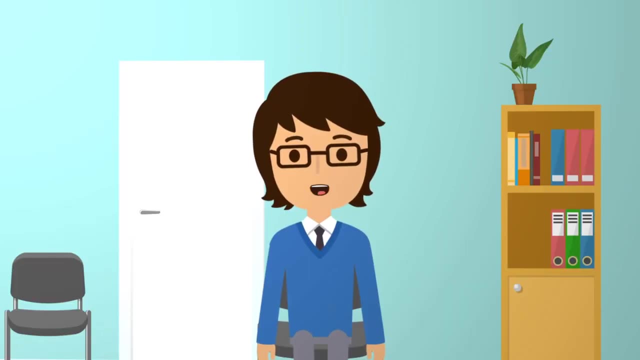 Can you help me understand? Kara recommended Ms Smith? Yes, Did Ms Smith stop her MAT program and for her to stop taking methadone while she was pregnant? Yes, of course. Our agency recommended that Ms Smith discontinue the use of methadone during her pregnancy. 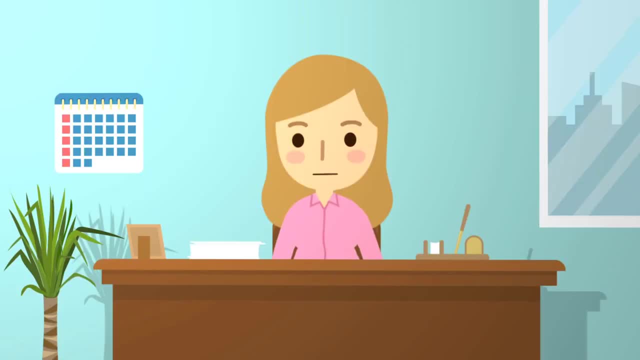 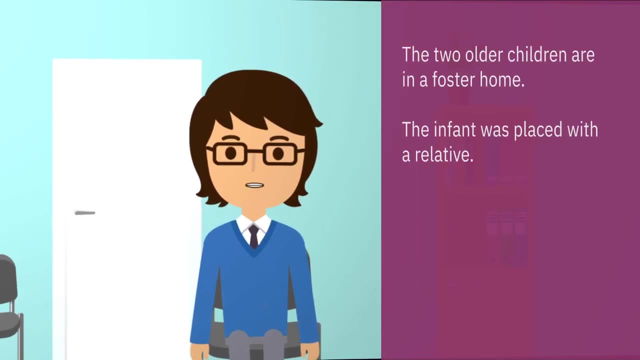 but not for her to stop attending her treatment program. Let's discuss this more. What services are in place for the family? I placed the two older children in a foster home and the infant was placed with a relative. We couldn't identify a relative able to care for all three of the children. 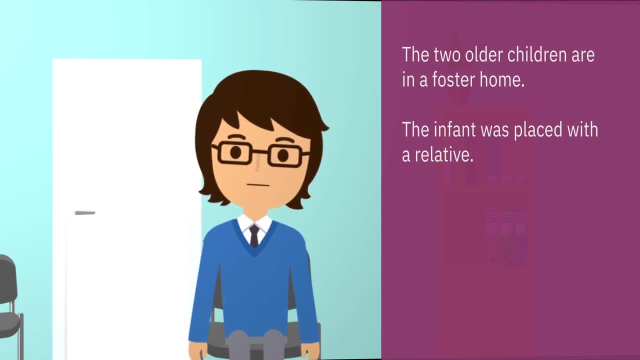 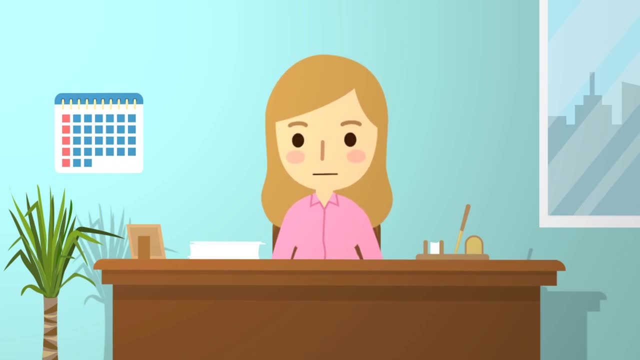 The relative's home study was completed and is attached to the court report. I've also initiated random drug testing. Have visitations been set up? yet One of the three children is an infant. I don't think Ms Smith should have visitation at this time. 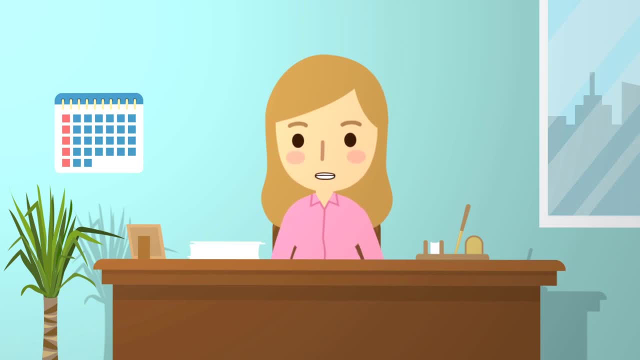 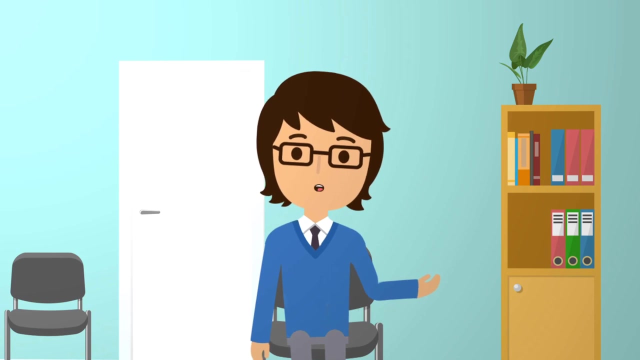 Why Ms Smith has the right to have visitation with all her children. I thought you shared that Ms Smith did receive MAT treatment services as part of her voluntary family services plan. Yes, But Kara, Ms Smith's previous ongoing worker, requested that she discontinue the use of methadone during her pregnancy. that was documented in her case plan. 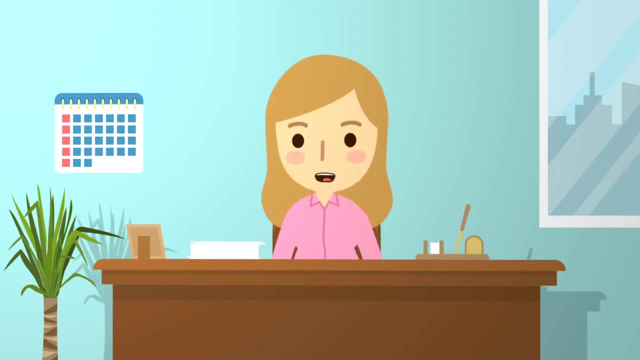 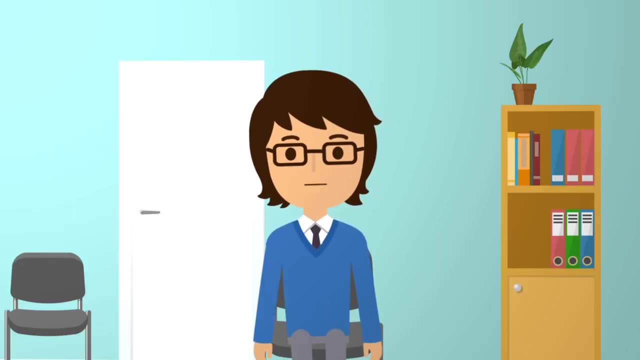 Ms Smith did not. Ms Smith was receiving methadone under the supervision of a licensed health care provider, right? Yes, and she received counseling at her program too. Did Ms Smith previously participate in random drug screenings? Yes, 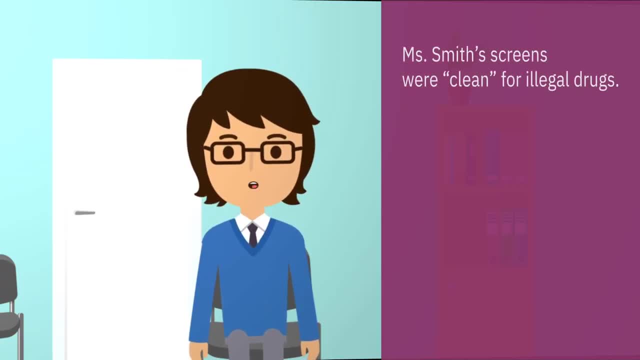 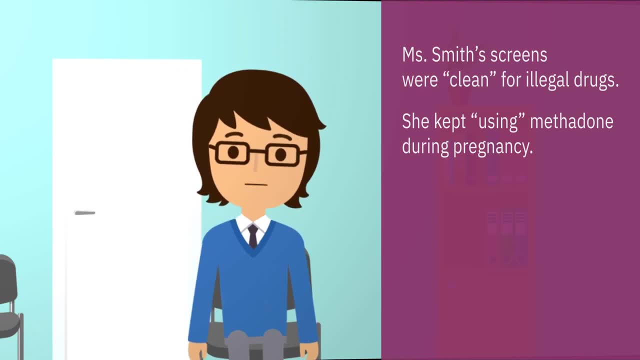 Ms Smith used methadone to break down. Ms Smith's screens were less whole and her Efx didn't run. but at her comfort, they 비� porec. Ms Smith spent two months holding it in herание, shot off the toxins and methadone injecting the baby. 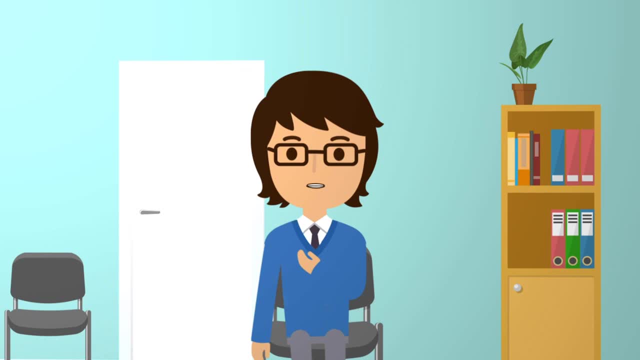 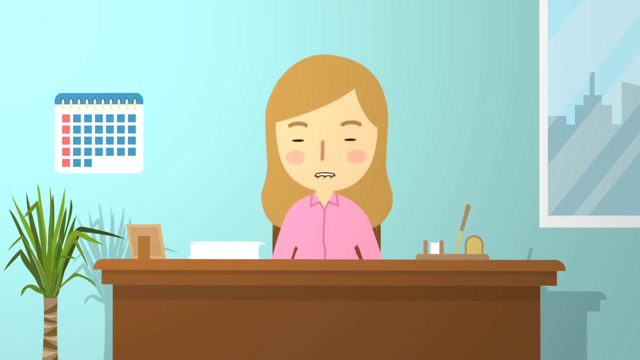 Ms Smith during her 比如 verwCO2.. prescribed dose of methadone does not mean that she is engaging in the illegal use of drugs. Kara would have a copy of her last random drug test so we can confirm it was only positive for. 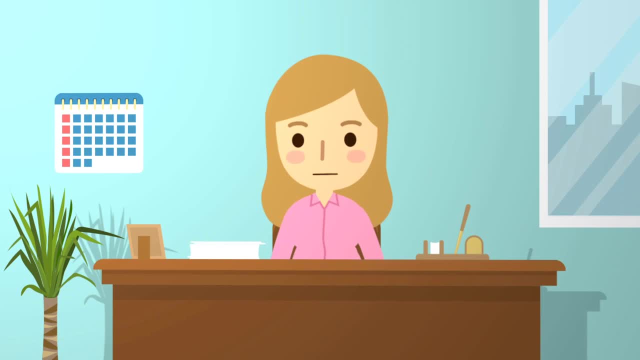 methadone? Do you have results of Mrs Smith's recent drug test? Yes, she was clean except for methadone. Did you attend the recent training on MAT and federal disability rights laws? No, Both were great trainings and I learned a lot about these laws and how they protect families. 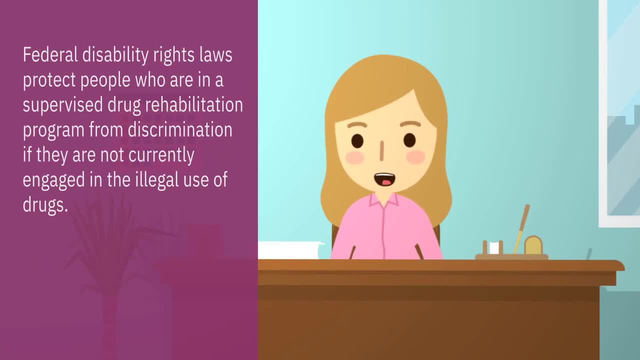 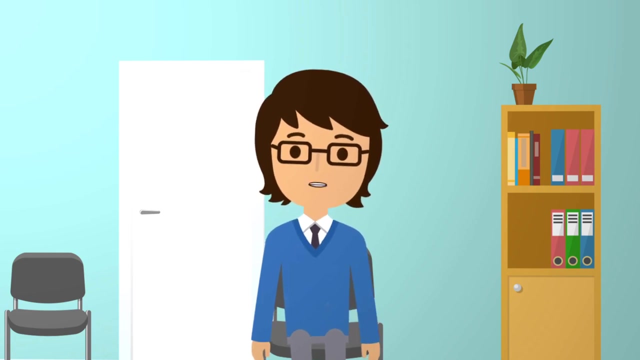 that we work with in the field. Did you know that federal disability rights laws protect people who are in a supervised drug rehabilitation program from discrimination if they are not currently engaged in the illegal use of drugs? Oh, this is new information to me. I guess I should sign up. 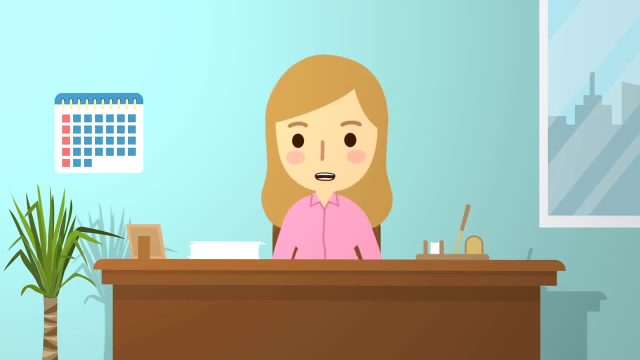 for the next class. Yes, I would like you to register for the next training. If you do, I would like you to sign up for the next class. If you do, I would like you to sign up for the next class. If you do, I would like you to sign up for the next class. 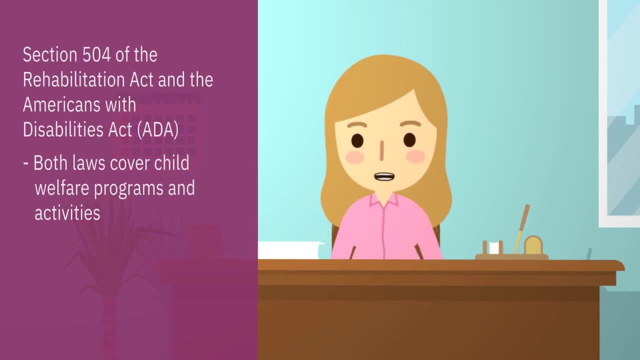 It will be a good opportunity for you to learn about Section 504 of the Rehabilitation Act and the Americans with Disabilities Act, because both laws cover child welfare programs and activities. I learned that methadone and buprenorphine are safe for use by pregnant. 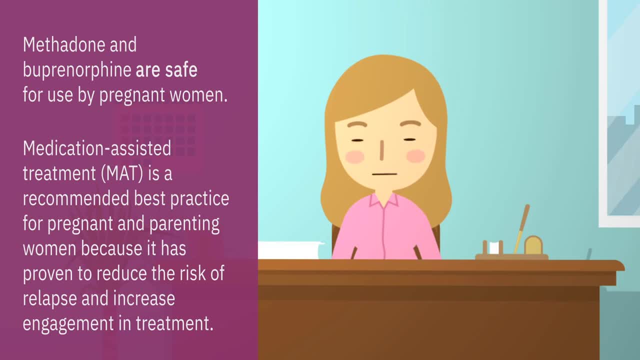 women. MAT is a recommended best practice for pregnant and parenting women with opioid use disorder, because MAT has proven to reduce the risk of relapse and increase engagement in treatment. SAMHSA's Division of Pharmacologic Therapies. part of the SAMHSA. 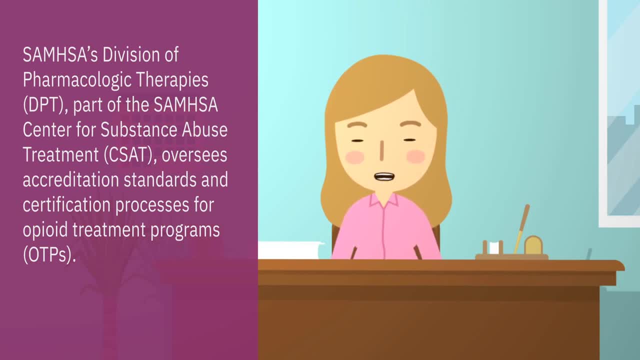 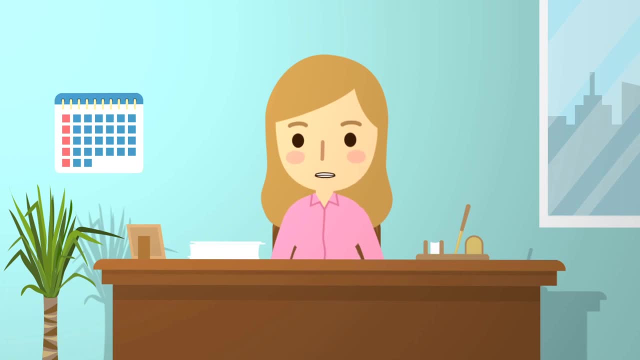 Center for Substance Abuse Treatment oversees accreditation standards and certification processes for opioid treatment programs. This is a good reminder for you, Ricardo, that recommendations and decisions that affect families and children must take several factors into consideration. Also, how a parent is progressing on the path to recovery is just 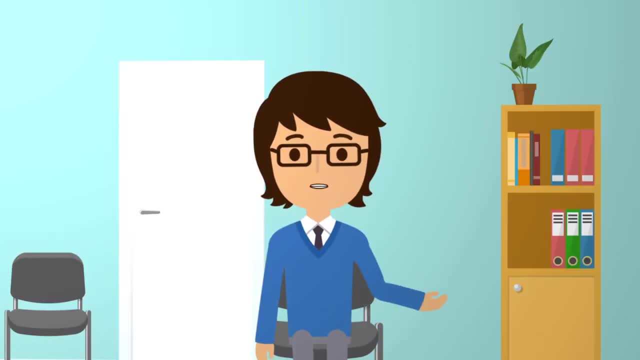 one of those factors. I have a question then. Ms Smith has prior substantiated allegations She was not able to supervise her children, has substance abuse issues and no family support. Wouldn't you remove the kids based on those allegations and her 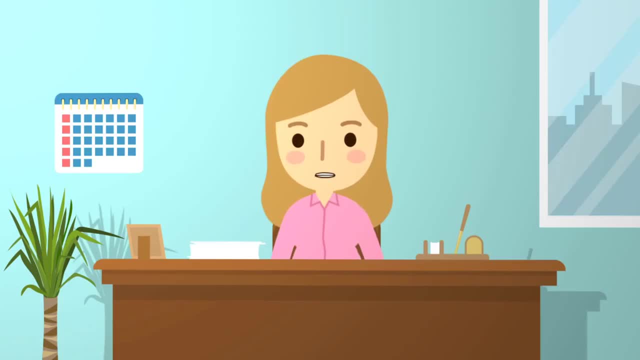 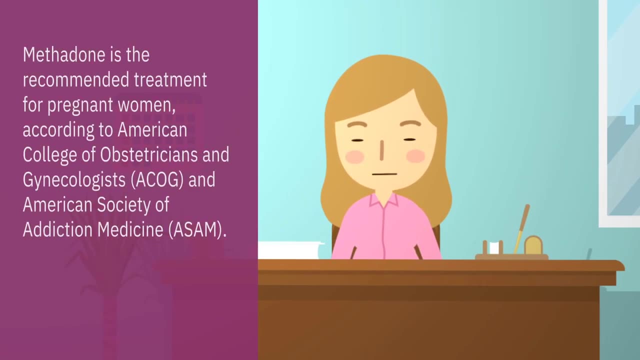 extensive CPS history. Instead of giving you a yes or no answer, let me tell you my concerns. Judgments were made about her continued use of methadone during her pregnancy. that did not factor in that methadone is the recommended treatment for pregnant women, according to. 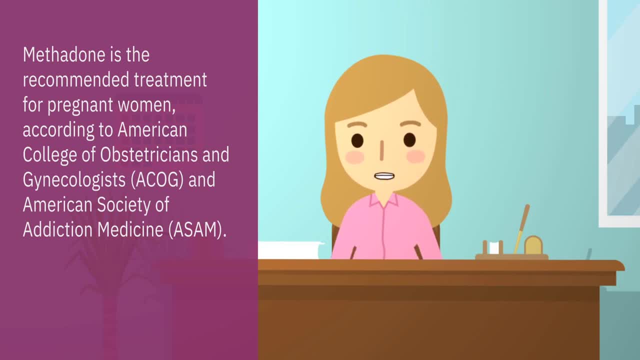 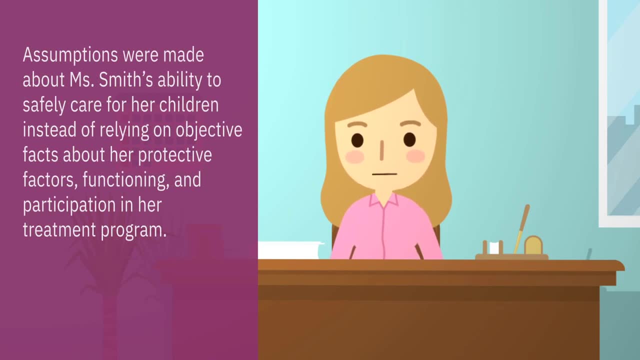 the American College of Obstetricians and Gynecologists and American Society of Addiction Medicine. Also, assumptions were made about Ms Smith's ability to safely care for her children while she is receiving methadone, instead of relying on objective facts about her protective factors functioning and participation in her treatment. 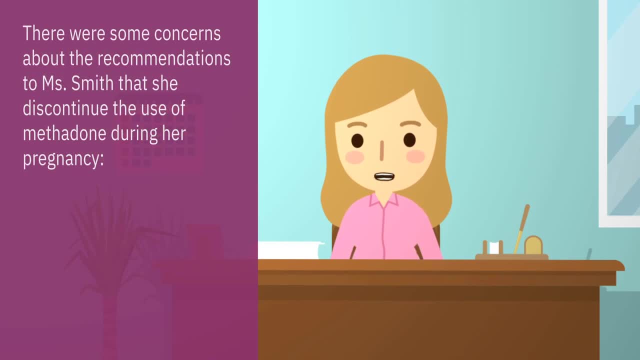 program. Additionally, I am concerned about the recommendations to Ms Smith that she discontinue the use of methadone during her pregnancy. Not only is that recommendation inconsistent with current medical standards, but it sounds like Ms Smith was treated differently from other parents because of her use of methadone. These facts 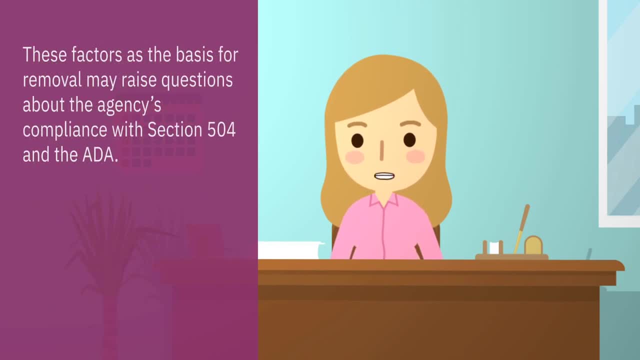 and factors as the basis for the removal may raise questions about the agency's compliance with Section 504 and the ADA. Also, I know that you are opposed to setting up visits between Ms Smith and her children, but we need to schedule visits immediately and a